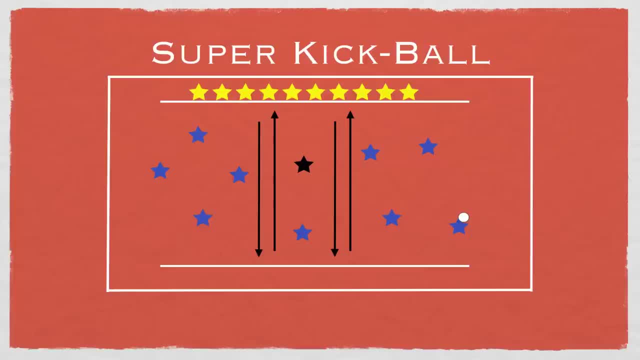 And they can get players out by tagging them with a ball or by throwing the ball at the players and hitting them as they run. They can also, if they catch the pop, fly. So if they catch the kick, that's one out. 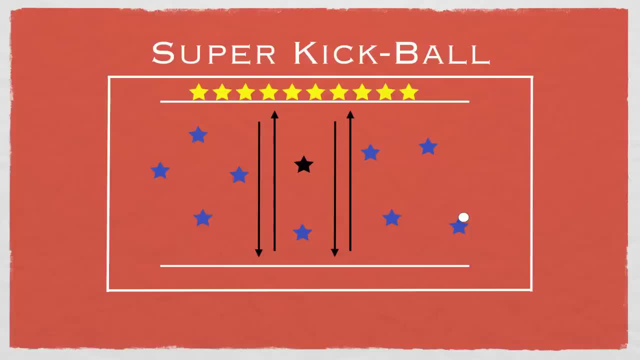 And if there are three outs, then the game ends. Also, the blue team can then choose if they want to pass it back to the pitcher or to the teacher. Once that happens, then players can no longer run, So whatever base they're on, they'll have to stay there and the game can continue on. And that's it for this idea. 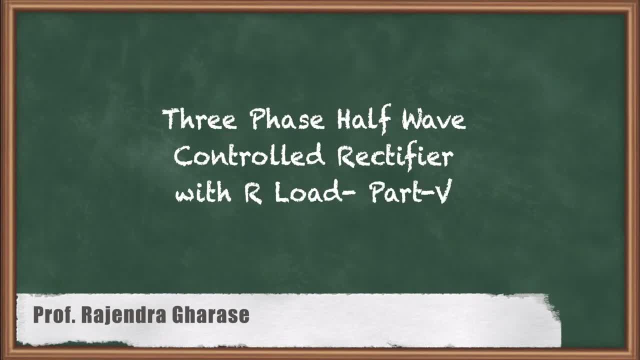 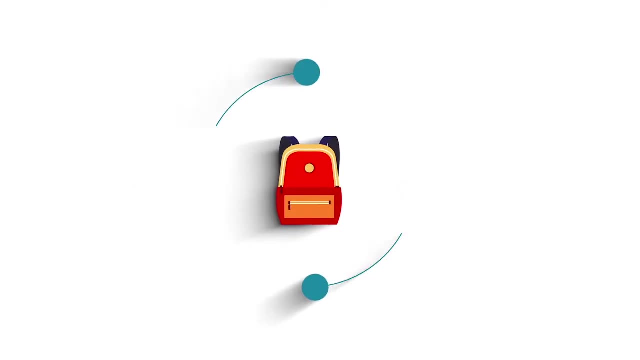 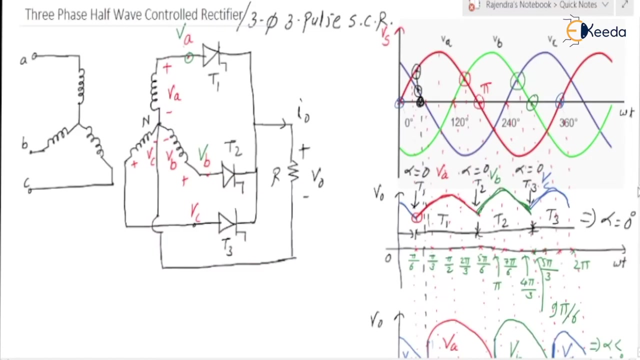 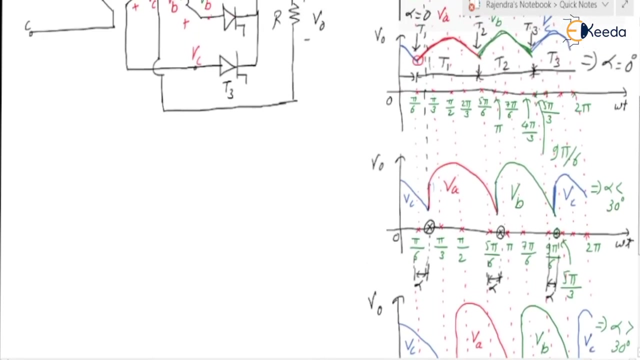 Hello friends, in this video we are going to derive the expressions of V0 average and V0 RMS for different values of alpha right for the three-phase half-wave controlled rectifier. Okay, so here we have already discussed about the V0 waveform for alpha 0, alpha less than 30 degree and alpha greater than 30 degree. okay, 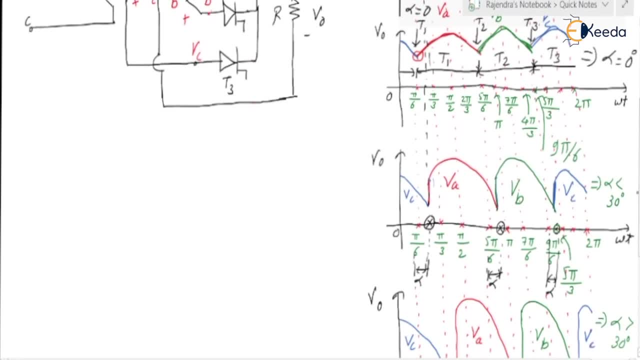 So if you check here, we are having the alpha equal to 30 degree is like a boundary condition. okay, So let us first derive the expression for V0 average and V0 RMS. okay for alpha less than 30 degree. 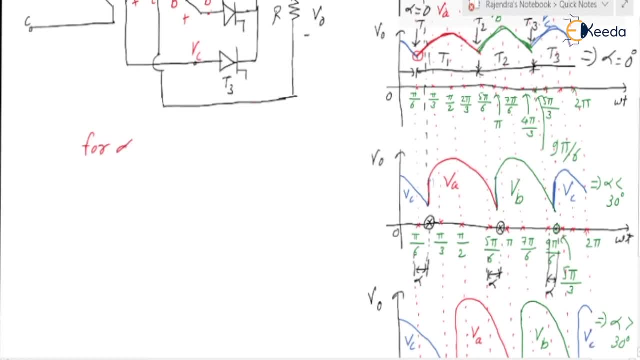 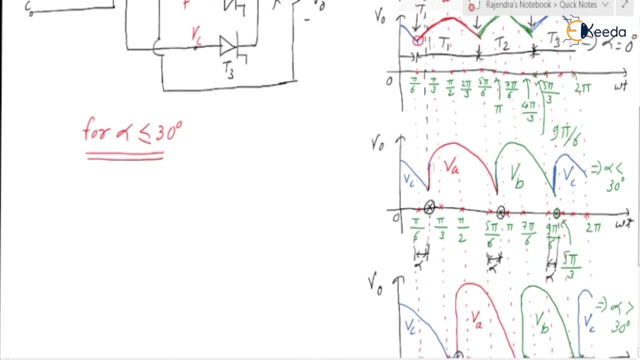 Okay, so please put the reading for alpha less than 30 degree, or we can write it as less than or equal to 30 degree. okay, Equal to 30 degree is for alpha equal to 30 degree. yes, both the expressions are valid, right. 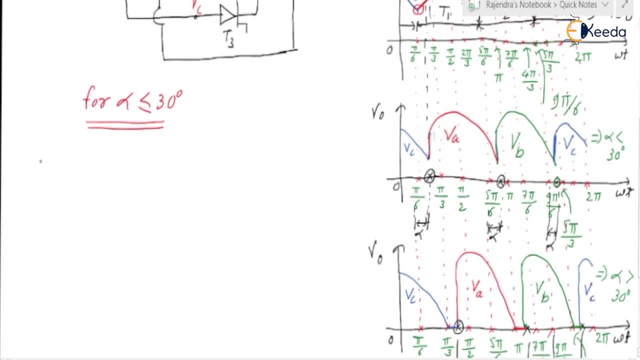 So here let us first write V0 average. okay, V0 average, yes, V0 average. So in the V0 average, if you check for alpha, less than 30 degree: yes, output voltage is VA, okay.